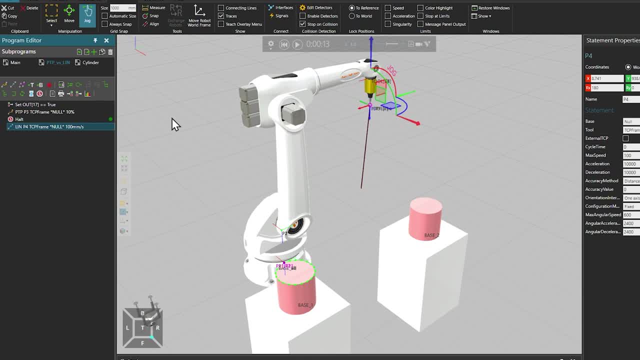 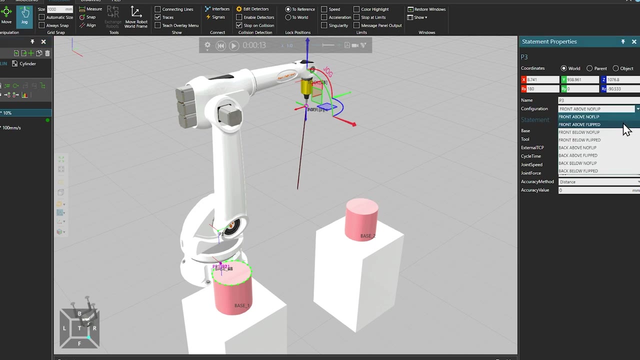 The difference between the motions is that with PTP it's possible to change the robot configuration, whereas with linear motion the configuration is retained. So in this case it's possible to change the configuration from a no-flip to a flip configuration. 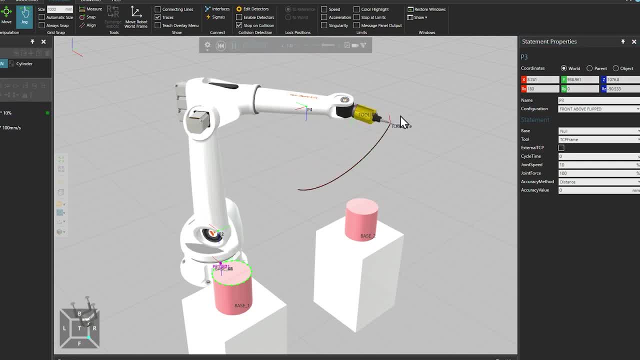 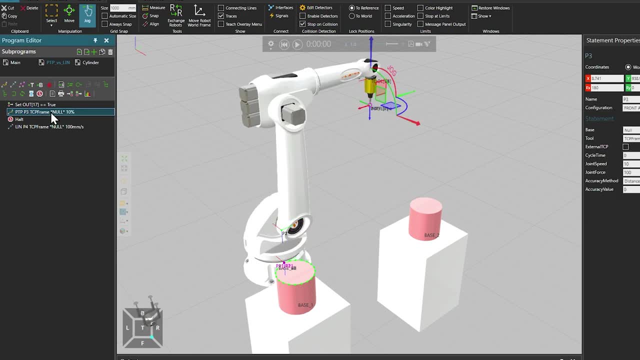 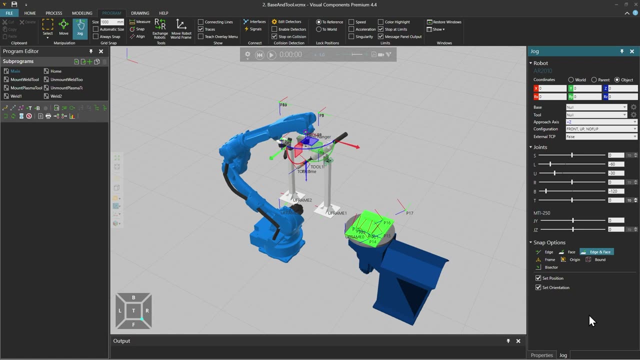 and you can see the wrist changing the configuration with PTP In your robot programs. you should always start with a PTP. And now let's talk about Robot Base and Tool Frames. Base and Tool Frames are important concepts to understand the positioning of your robot. 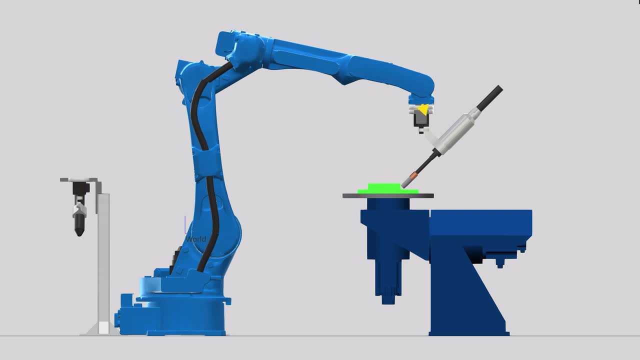 A tool frame sets the location for the tool center point, or TCP. In this illustration it's the yellow arrow from the robot flange to the end of the welding gun where the TCP is located. A base frame is the reference frame for positioning the TCP. 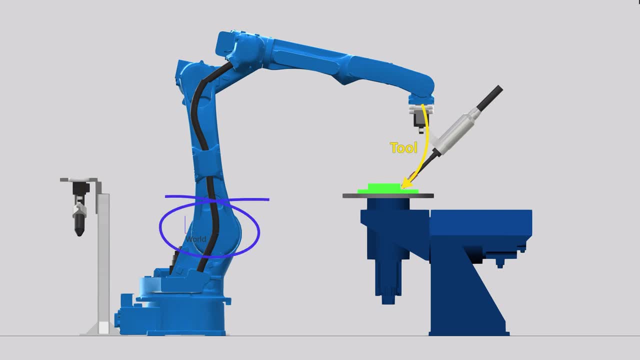 By default it's at the robot world frame, but you can move it, for example, to the corner of a workpiece or fixture. And now, when you program positions, the target position matrix will be the transformation from the base frame to the TCP location. 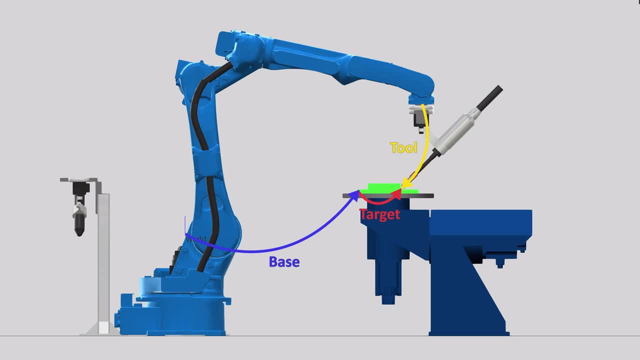 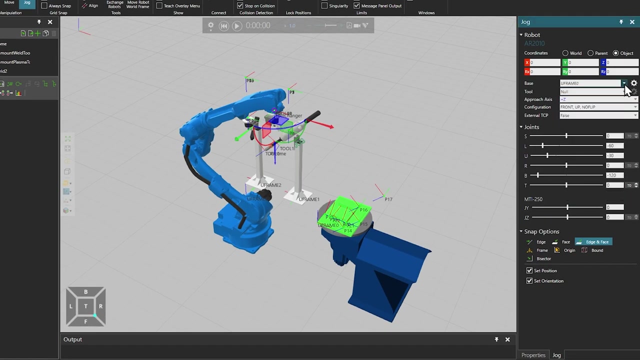 And together the chain of base, target and tool form this combined transformation called Robot illustrated here, And that transformation is passed to the robot kinematics to solve the joint values for this given TCP position In Visual Components you can set the active base and tool frames in the jog panel. 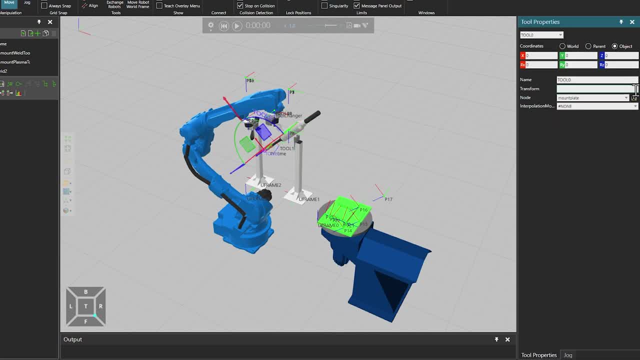 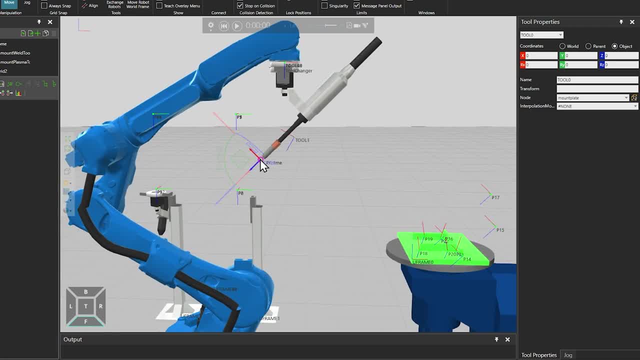 And you can modify the frames by clicking the gear icon next to the frame. When you modify the frame you can set its location and you can also set the parent node to be some simulation component or node in the layout. So setting the parent for a frame attaches the frame to certain components in the layout. 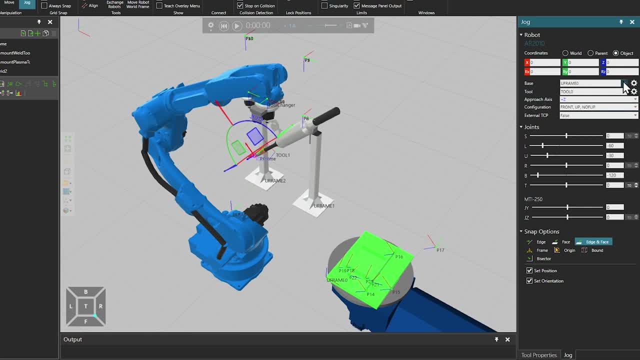 Visual Components. robots usually have 16 built-in base and tool frames, but you can also import frames from the layout. But you can also import frames from the layout. But you can also import frames from the layout. For example, we can export tool frames from attached components. 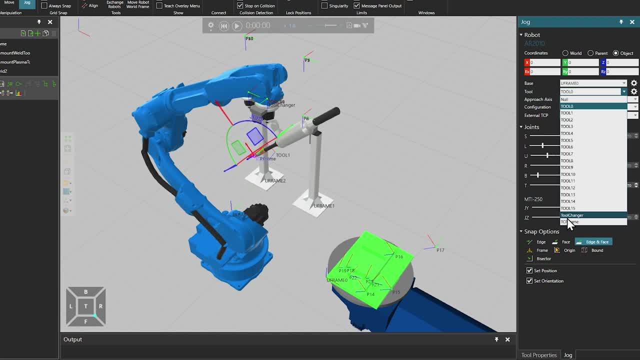 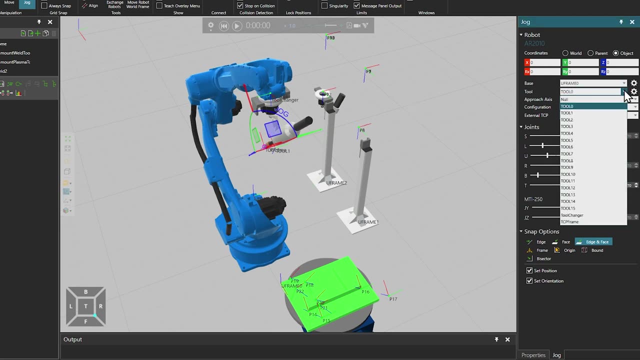 via the interface behaviors for Tool and Robot Positioner. So in this example there are two imported toolframes from the connected components. Many times for the toolframe you only need one, but there may be cases where you need multiple toolframes. 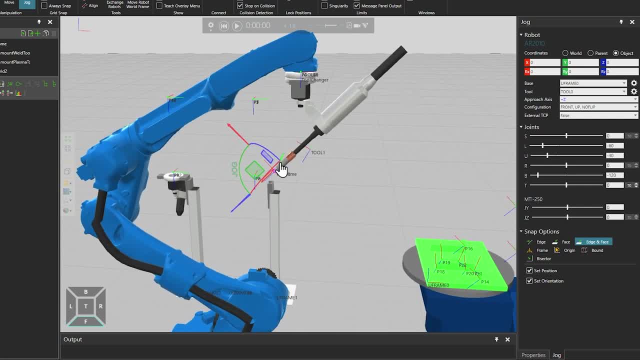 For example, in this layout we have a weld gun on the robot. For example, in this layout we have a weld gun on the robot. For example, in this layout we have a weld gun on the robot, on the robot, and we are using the first tool frame for that tool component. but 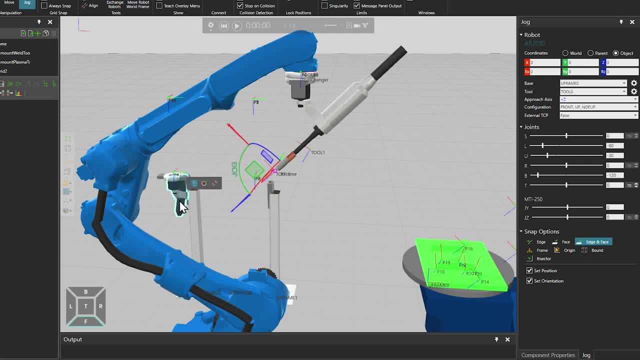 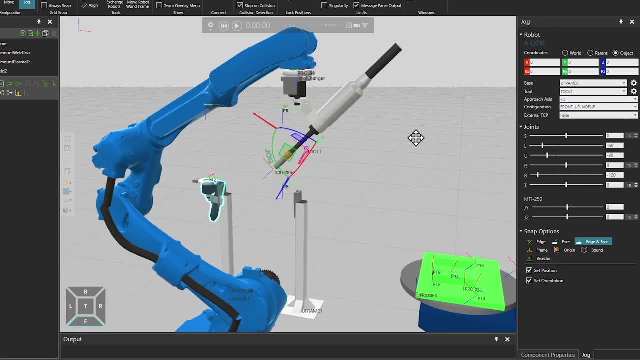 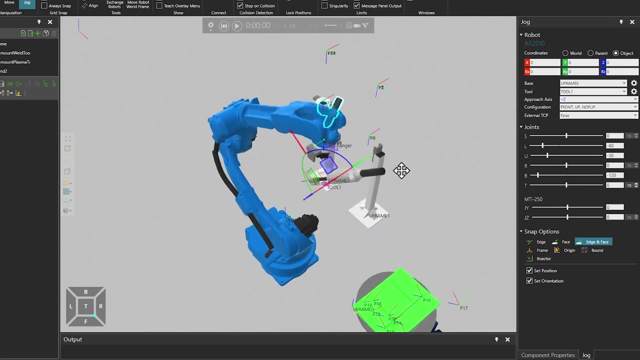 we also have a second tool for plasma cutting where the geometry does not match the first tool frame. so we need a second tool frame position here that will match the geometry of the second tool component. so what are the use cases for robot base frames? usually you attach base frames to 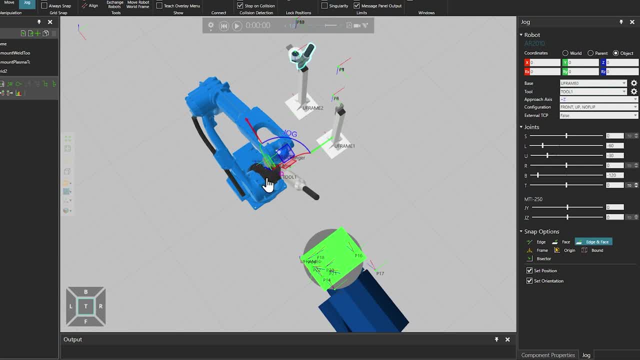 certain components in the robot cell which the robot needs to move to. in this example, the robot works on the workpiece and we have one base frame for that, but the robot also needs to work on this pair of tool stands. so in this case we have a second and third base frame attached to the tool stands. 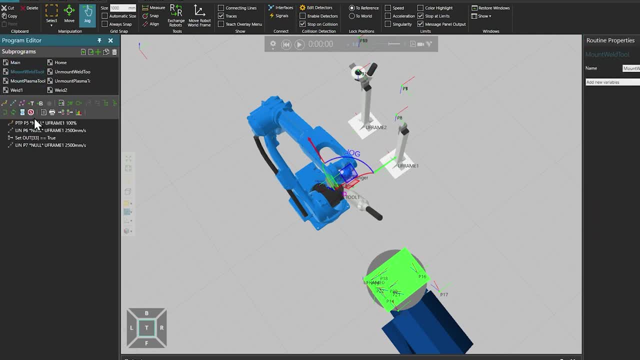 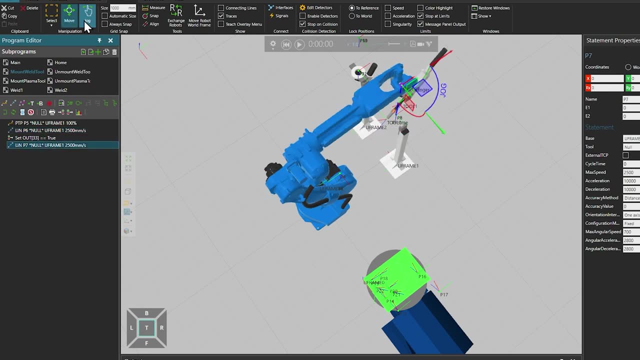 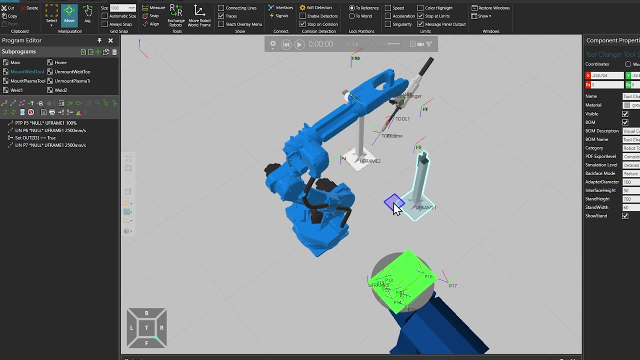 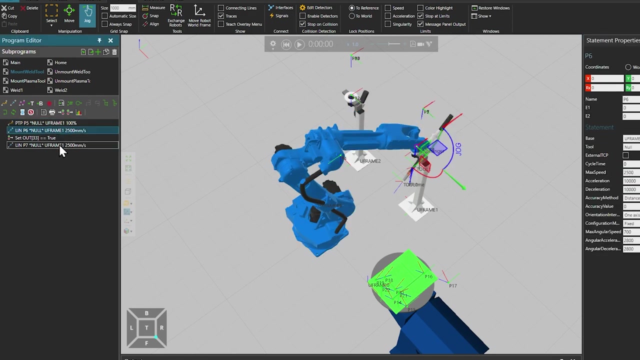 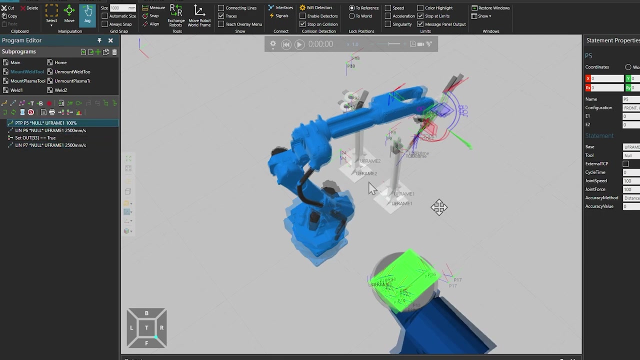 for example, the weld tool uses the first tool- stand and base u-frame one- and when the base is attached to the stand, if we need to modify the position of the stand, we don't need to modify the program for picking the tool on that stand, because the positions move with the base frame that is attached to the component. 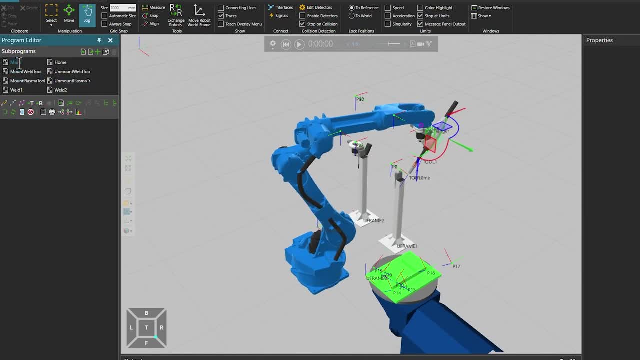 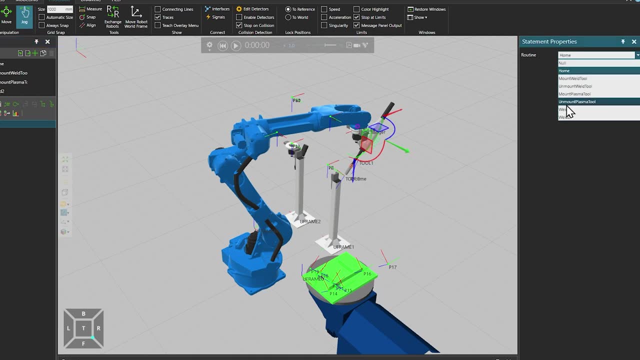 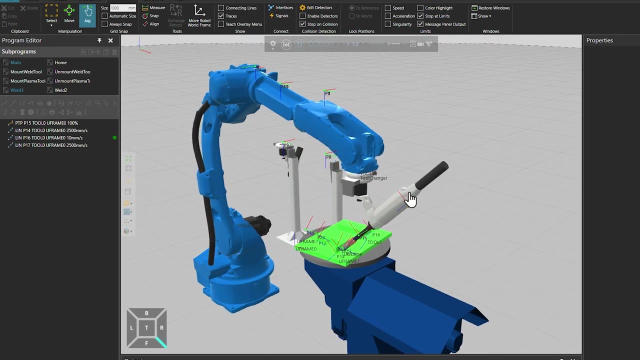 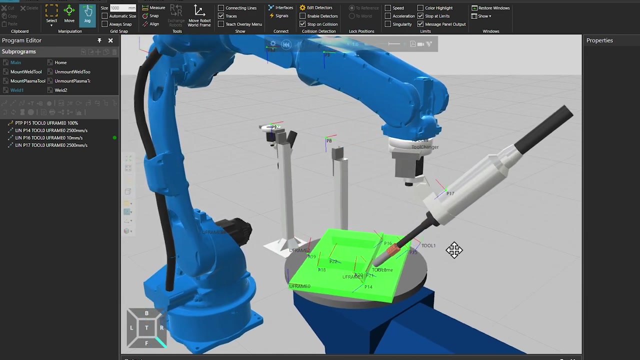 a base frame is also useful if you need to perform synchronized motions. so in this case we have a weld one routine set to weld on this edge while the workpiece is moved by the workpiece positioner, and this is synchronized motion. that is possible by using a base frame. 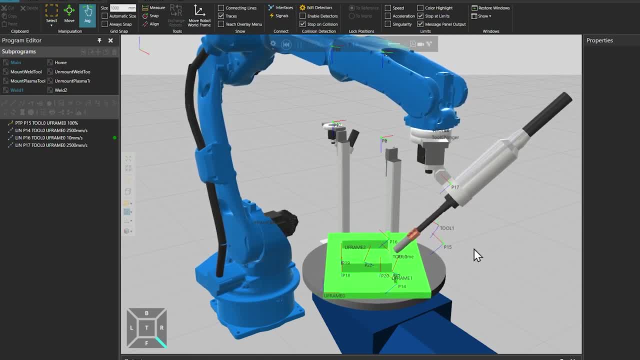 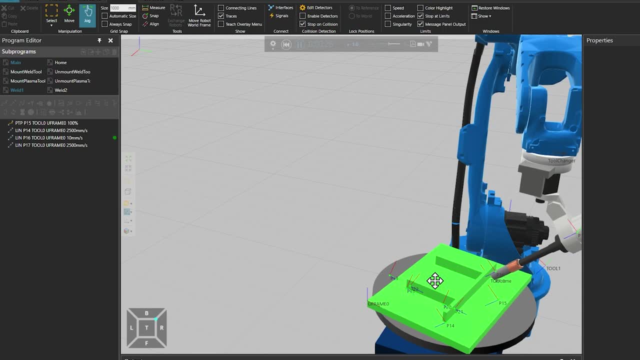 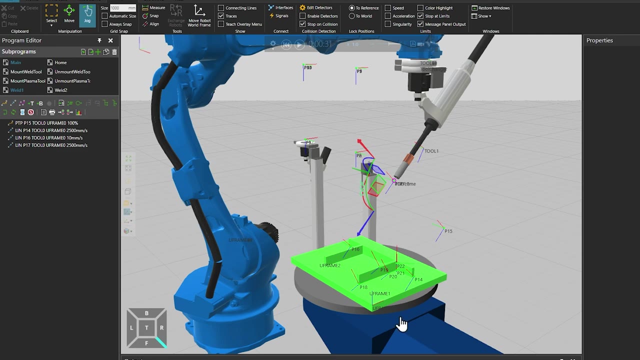 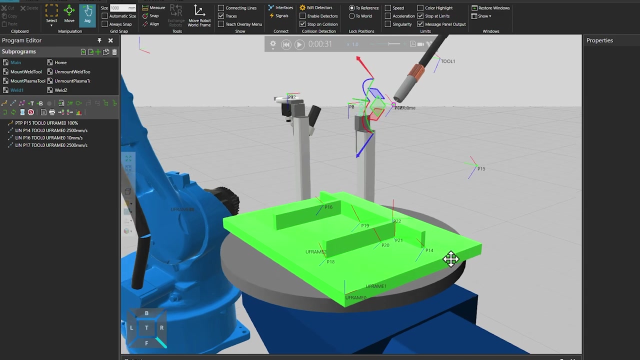 and in this case, the base frame needs to be attached to the moving workpiece, or you could set the parent to be the flange node of the workpiece positioner. and now, when the workpiece moves, the robot performs a linear motion in reference to the moving base frame. 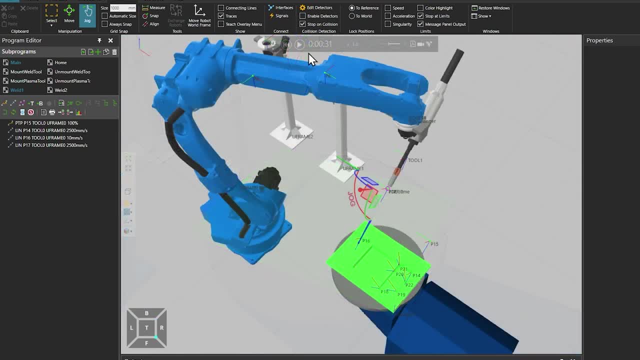 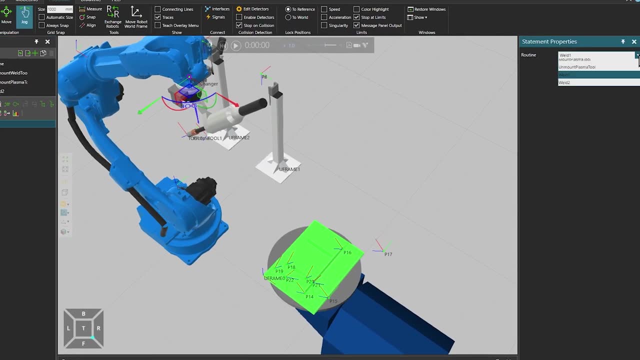 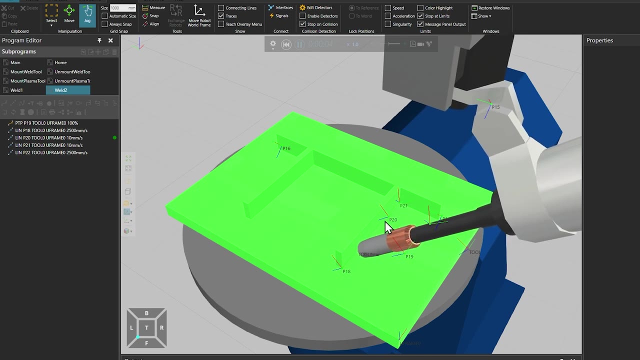 another use of base frames is reusing your programs and creating patterns. so here the weld, two subroutine welds this edge of the workpiece and in this example we have another similar feature on the workpiece. so we could reuse the program for the second instance of this stiffener feature. 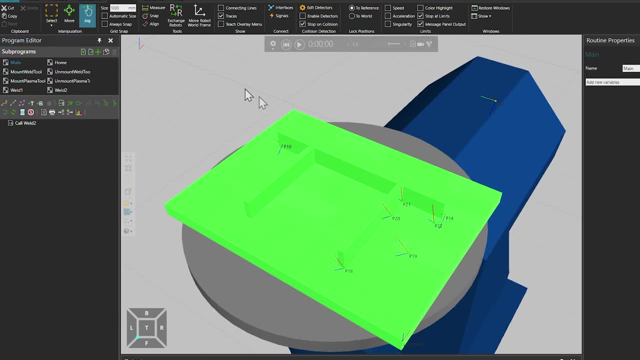 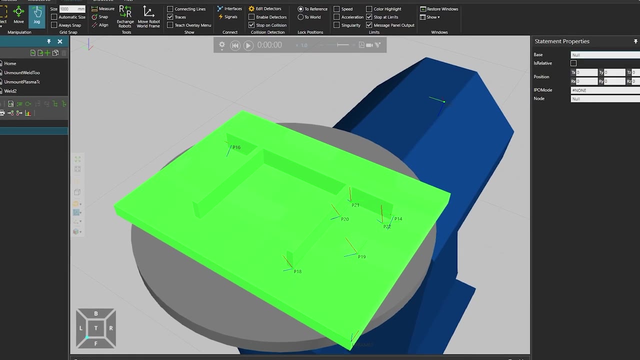 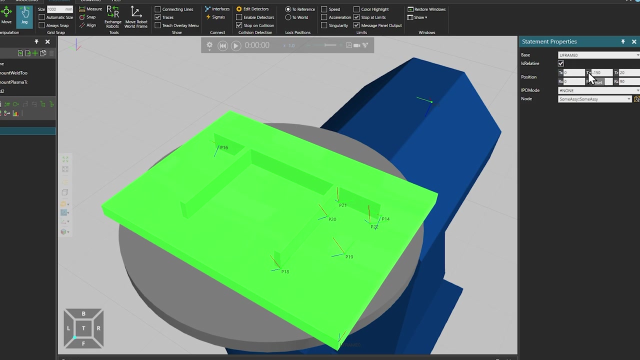 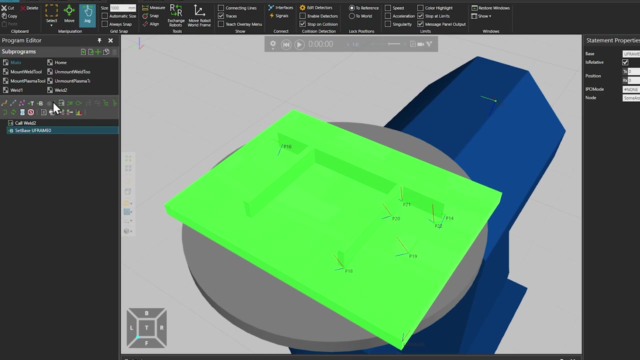 and that we can do by modifying the base frame. so if we do a simple measurement, there's 160 millimeters offset between the similar, stiffener features and what we can do is modify and move the base frame relatively by that amount and then we can call the weld two subroutine again. 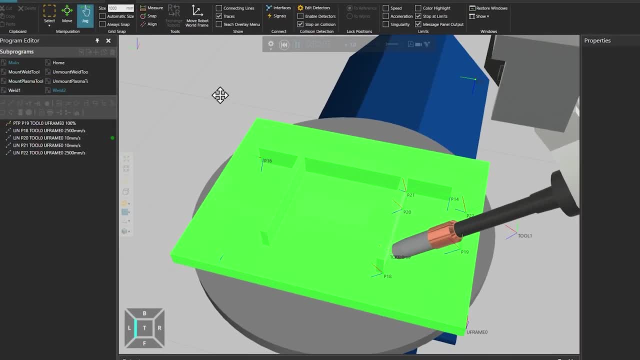 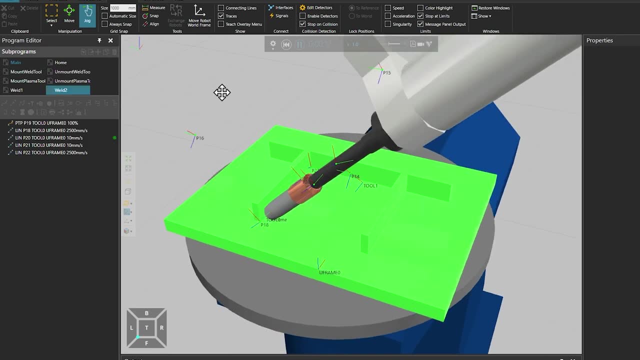 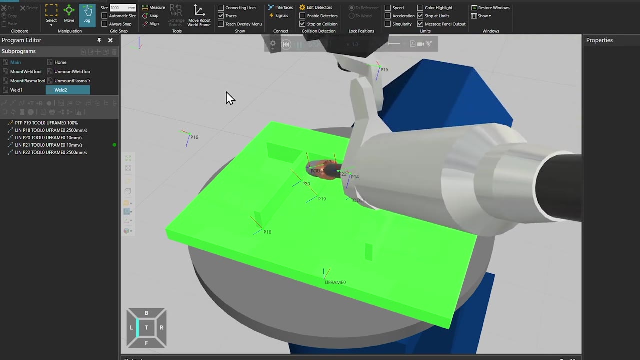 and what happens then is that the robot welds the first feature switch in the same way and then it moves the base frame 160 millimeters and repeats the same routine to weld the second feature on the workpiece. switch ons, switch off as long as it moves suddenly, after also applying the motion to a chamber and anyone at the 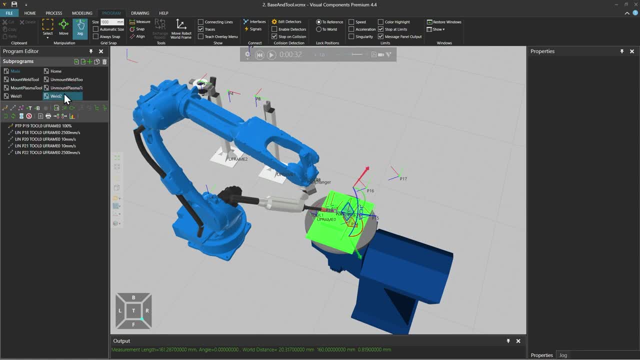 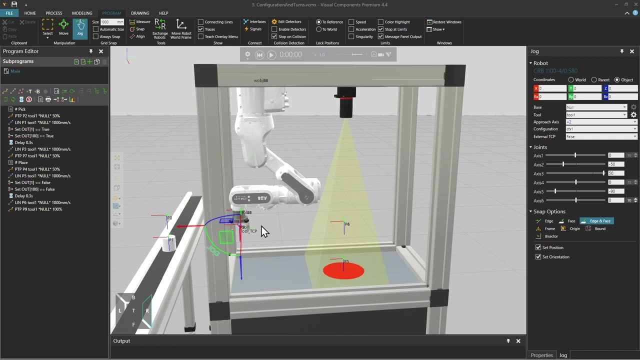 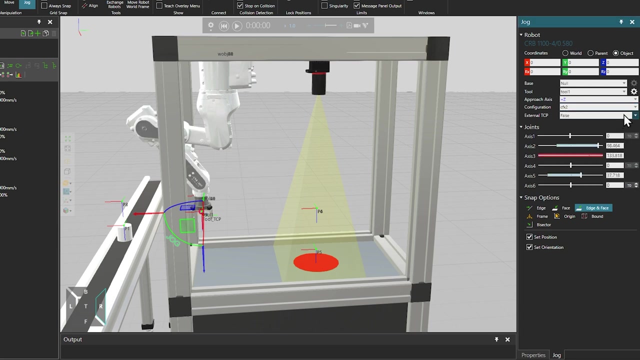 programs. it's easy to create patterns and re-use your programs on another instance. And now let's talk about robot configurations and joint turns. Configurations are different ways for a robot to reach the same tool position, And an articulated robot has 8 of these configurations that you can select from the jog panel. 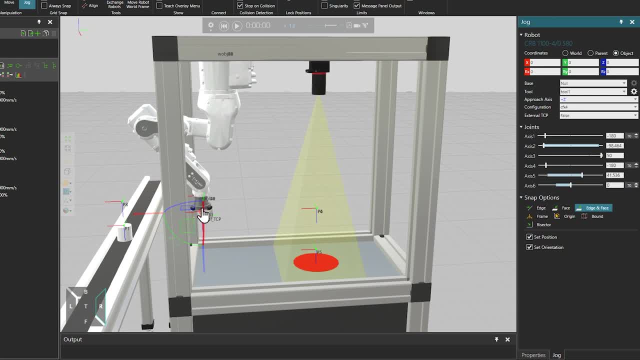 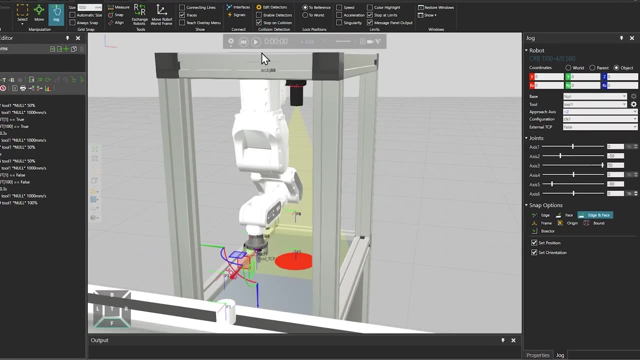 Selecting different configurations shows that the tool stays in place, but the robot pose changes And sometimes you need to use all of these different configurations in your applications. So let's take a look at this example layout. If we run the simulation, the robot picks up the part and places it under the camera. 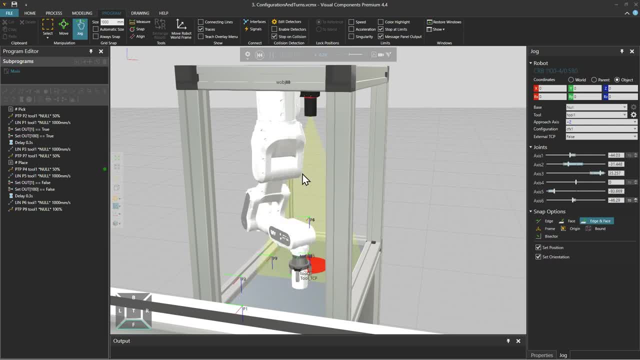 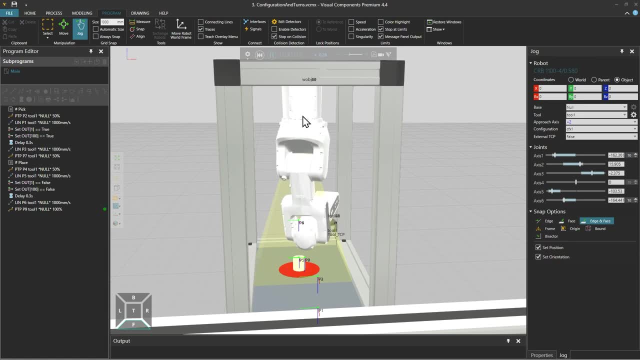 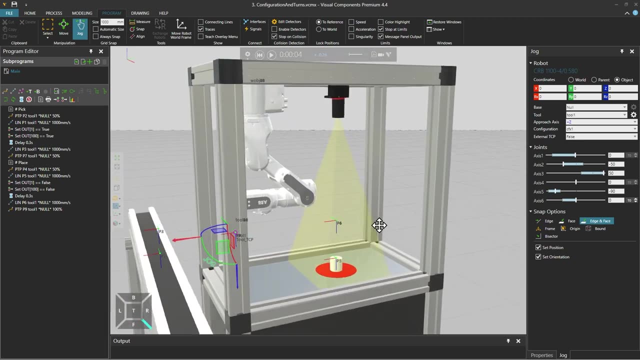 using only one configuration, And this means that in this case, The robot's first axis needs to rotate, causing the wrist to hit the structure of this narrow cell. So what we can do is change the robot motions to use a different configuration to reach. 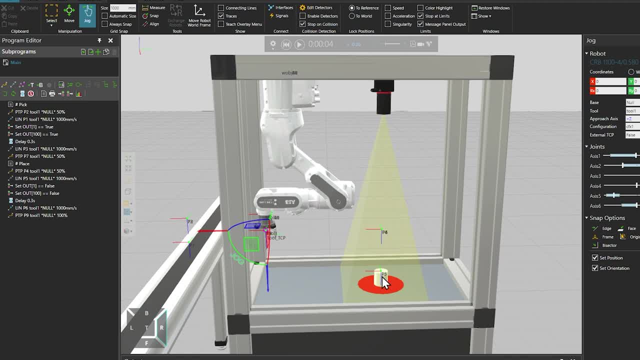 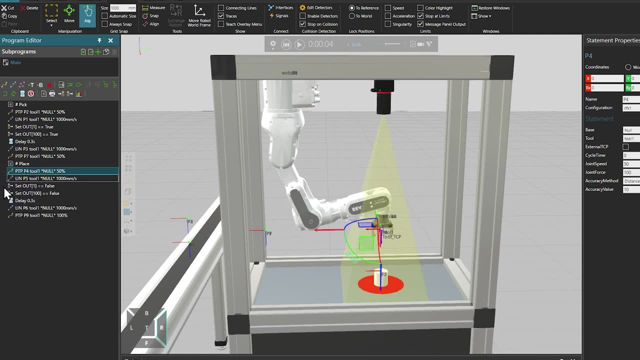 the camera location You can change the configuration on a robot's PTP motions And all linear motions that follow. it will inherit the configuration from the PTP motions. So in this place position, let's select the last PTP motion and change its configuration. 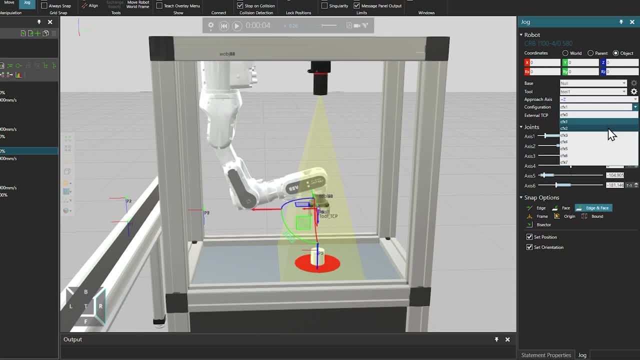 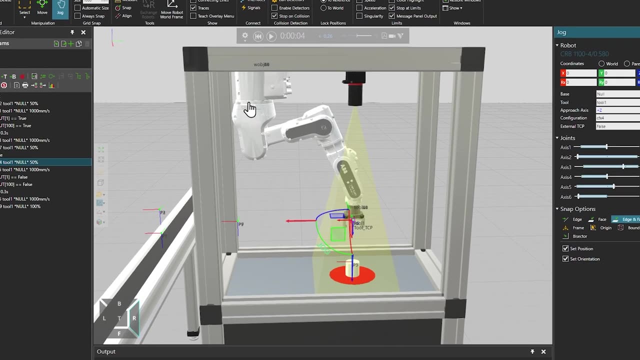 using the jog panel, And here we want to set the configuration so that the first axis stays close to the zero position, And in this case, this configuration- CFX4, is the one we want to use. So we use the touch up function on the position. 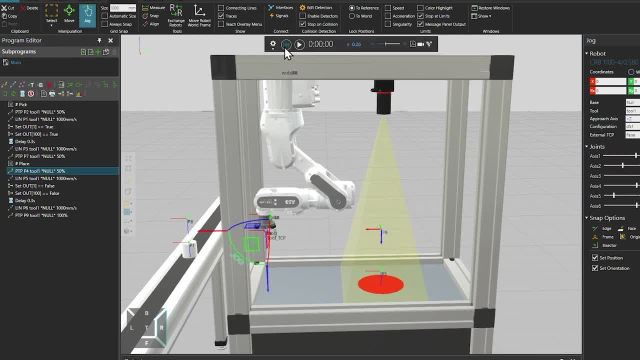 And with the up position, The updated configuration lets run the program now. Now you see that the robot doesn't turn on this first axis anymore, But axis 2 and 3 do most of the work to arrive to this camera position. So we used a different configuration to optimize the robot motion. 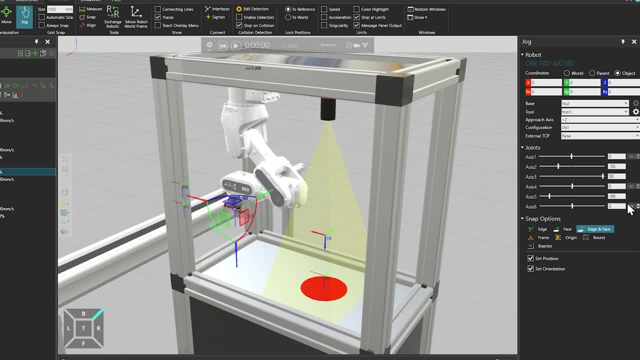 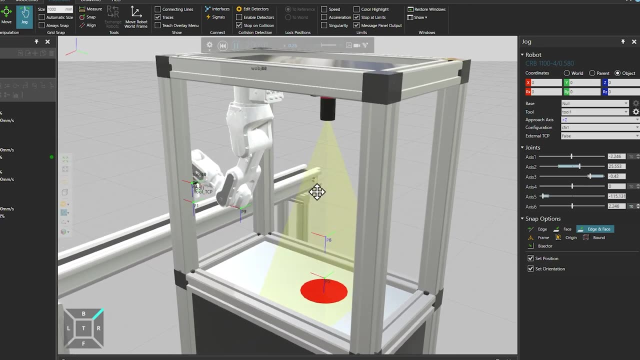 Joint turns are related to robot configuration In that with a rotational joint you can have different full rotations programmed to some position. And if we take a closer look at this program you can see that the robot picks the part and when it approaches the sixth joint does a full rotation when arriving to the camera. 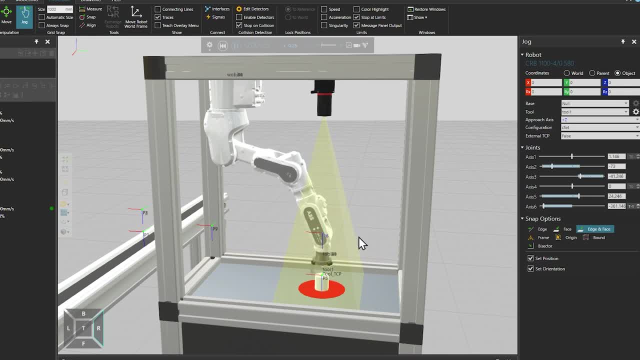 position, And this is unnecessary motion that we can fix by modifying the joint turns. So, again, we can see that the robot is now in the position of the camera And we can see that the robot is now in the position of the camera.